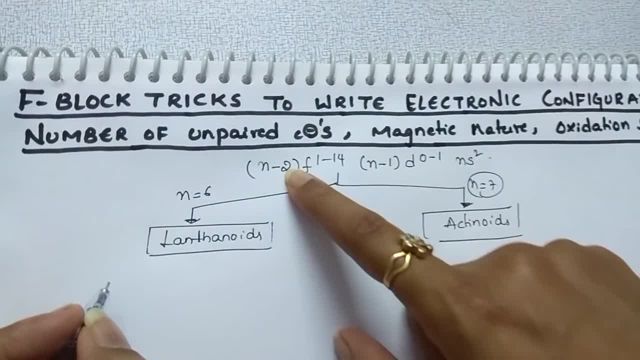 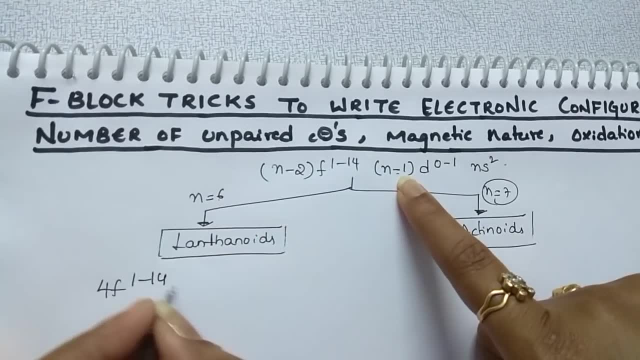 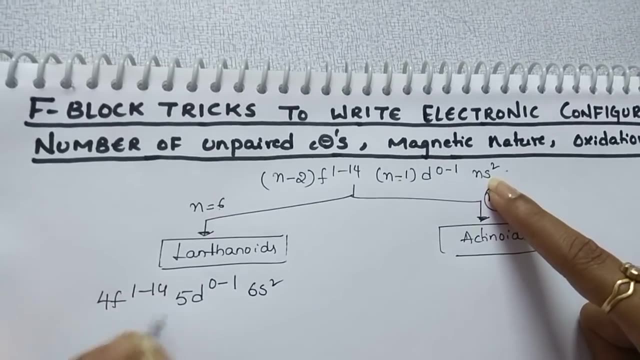 value of 6 in this general formula: 6-2, 4, F, 1 to 14, 6-1, 5, D. it may have 0 to 1, 6, S2.. This is the general configuration of lanthanides Coming to the actinides. what is the N value? 7,. 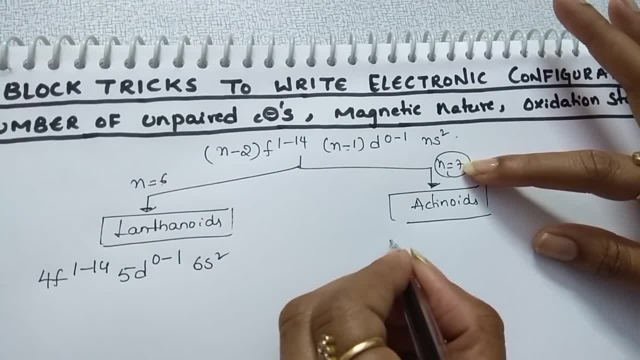 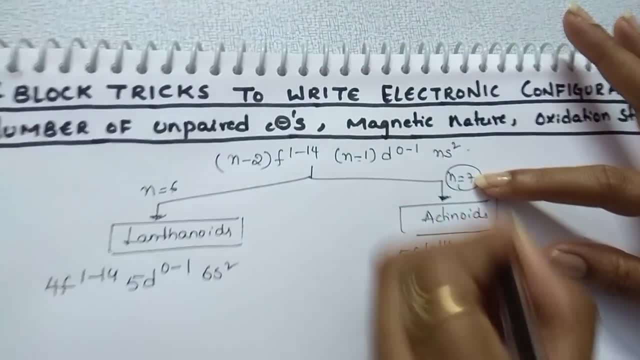 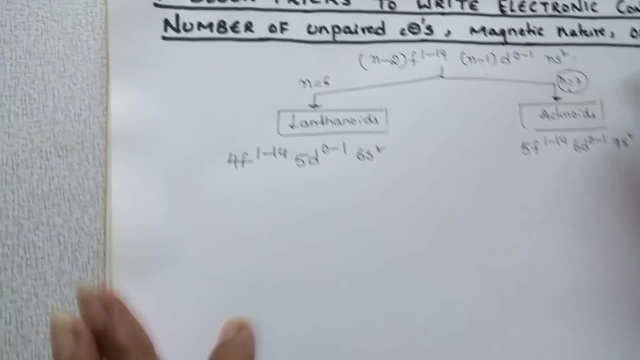 substitute the value of 7 in this formula: 7-2, 5, F, 1 to 14, 7-1, 6D, 0 to 1, 7, S2.. This is the general electronic configuration of actinides. Let us see first for lanthanides. 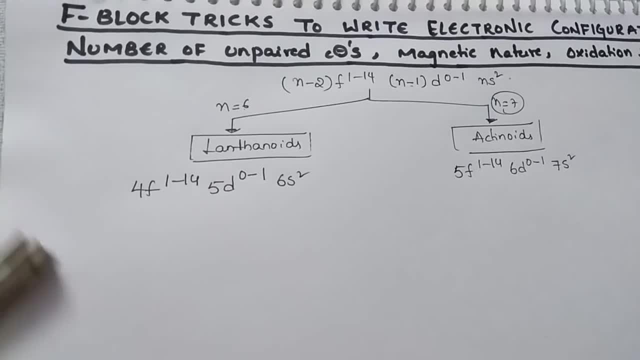 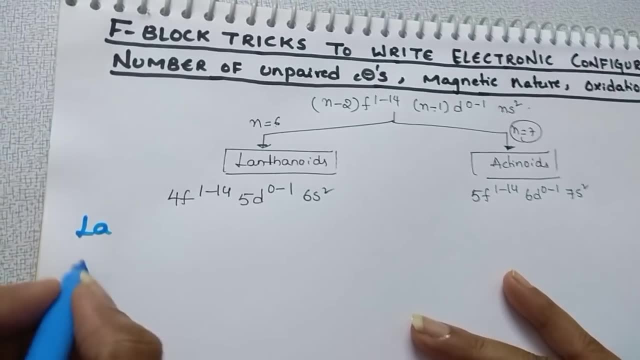 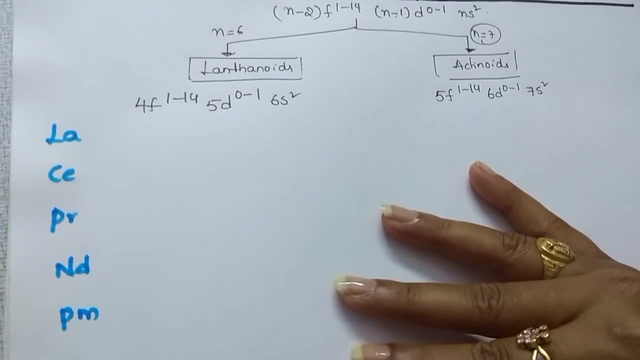 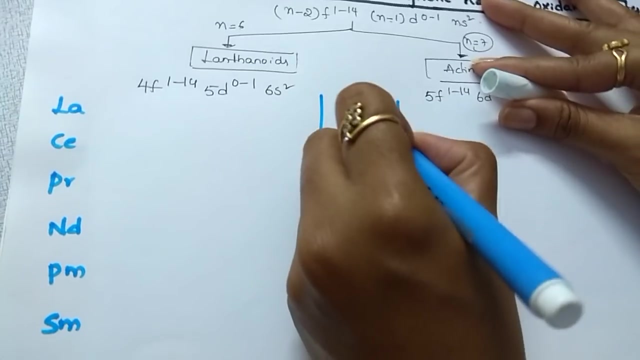 By using this trick, you are going to find the electronic configuration. I am going to write the element: Lanthanum, cerium, praseodymium, neodymium promedium, samarium europium gadolinium terbium. 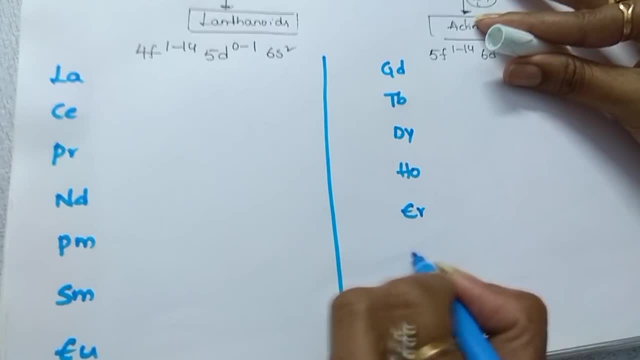 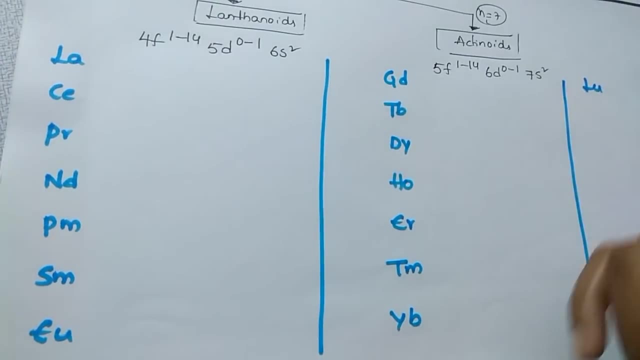 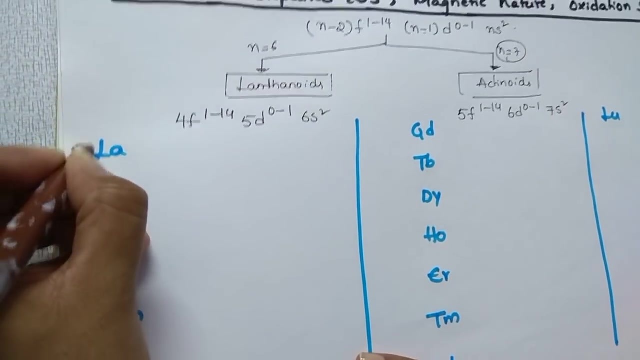 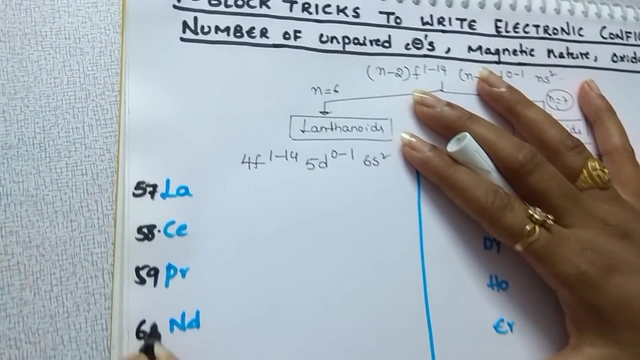 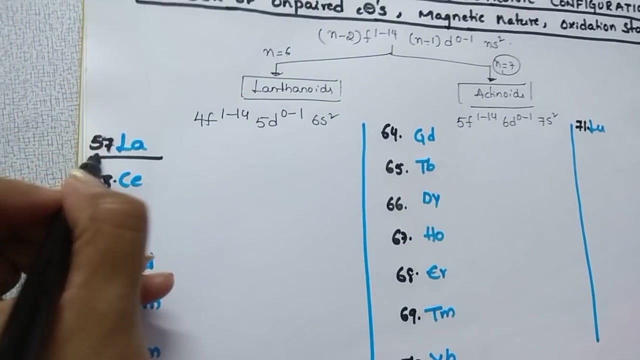 disposium holmium, erbium, thulium, iterbium lutetium. These are the lanthanide elements. Atomic number of lanthanum is 57.. Cerium 58,, 59. Means after lanthanum, means with atomic number 57.. 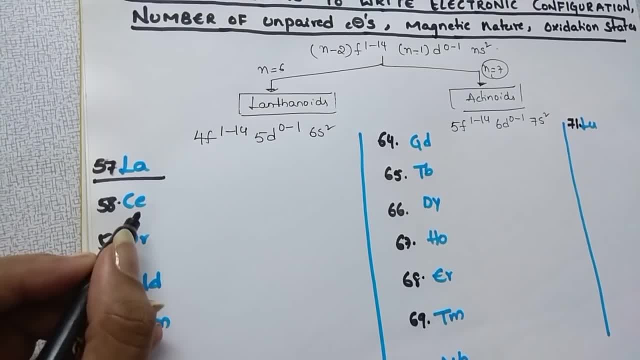 After lanthanum, from atomic number 58,, that is, cerium, to atomic number 71,, lutetium. these elements we call it as lanthanides, Lanthanides, Lanthanides, Lanthanides. 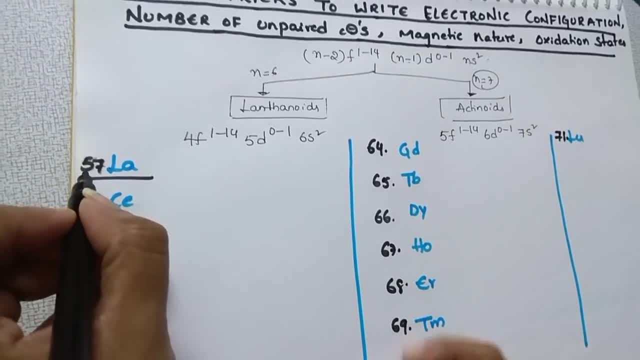 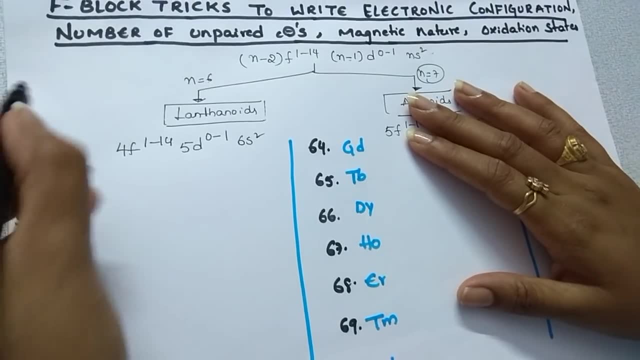 Lanthanides, Lanthanides, Lanthanides. After lanthanum, we call it as lanthanides, Atomic number 57.. So what is the nearest noble guess of atomic number 57 is xenon, with atomic number 54.. 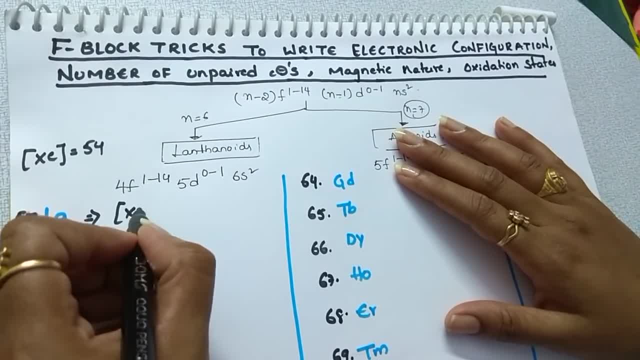 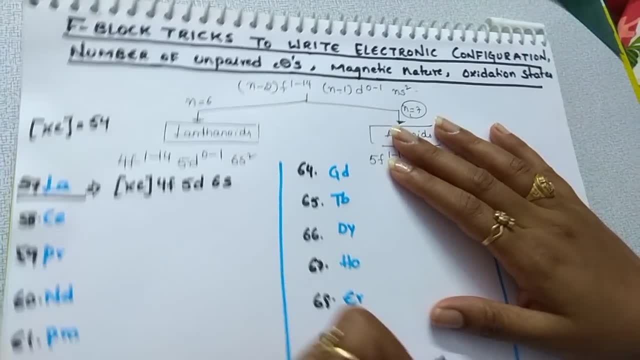 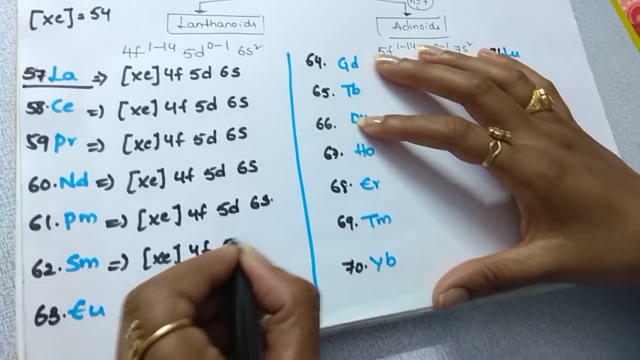 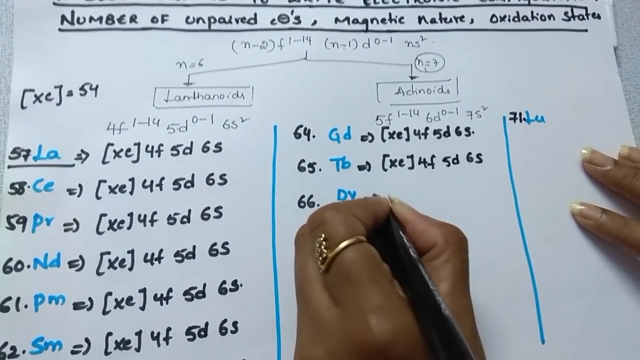 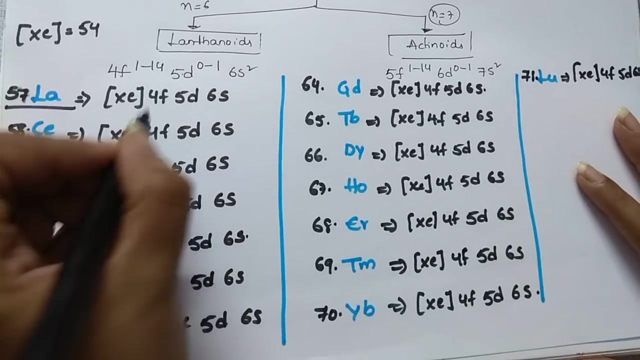 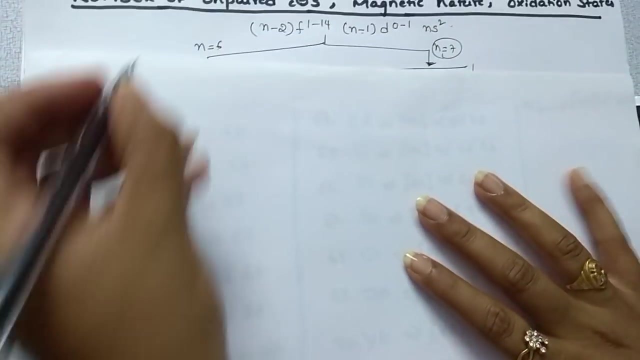 Right. So what I am doing is first write xenon, after that 4F, 5D, 6S, Clear, Just I am going to write this same thing for all the elements. So, after writing xenon- 4F, 5D, 6S- what you have to do is just take the numbers from 1 to 14.. 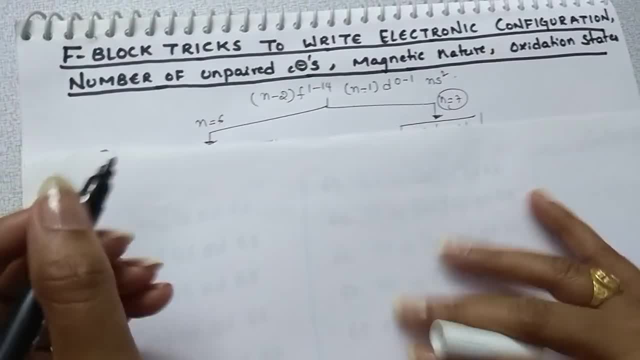 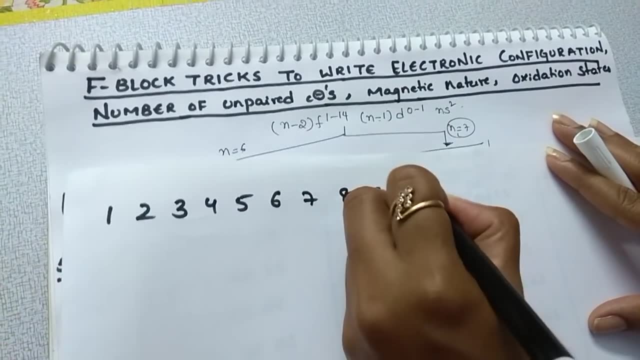 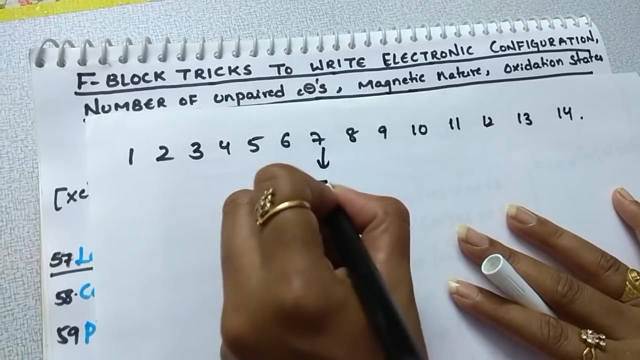 Because F can accommodate a total of 14 electrons, So 3.. 4,, 5,, 6,, 7,, 8,, 9,, 10,, 11,, 12,, 13,, 14.. And in F, half filled is 7 and completely filled is 14, which is more stable. 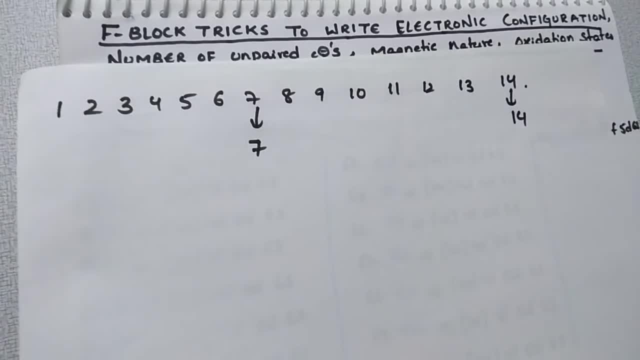 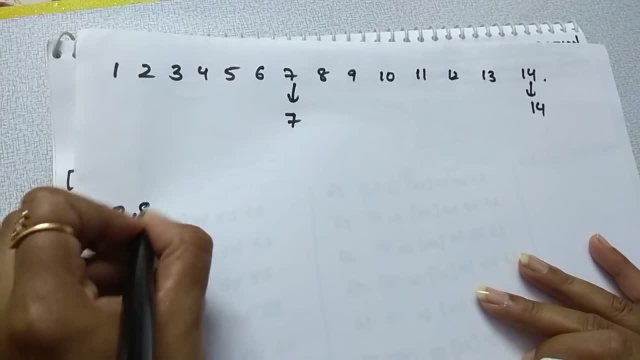 So there is no change in the configuration of these two. 7 and 14 are more stable After that. the numbers you should not take is 2 and 8.. 2 and 8.. 2 and 8.. For lanthanates. 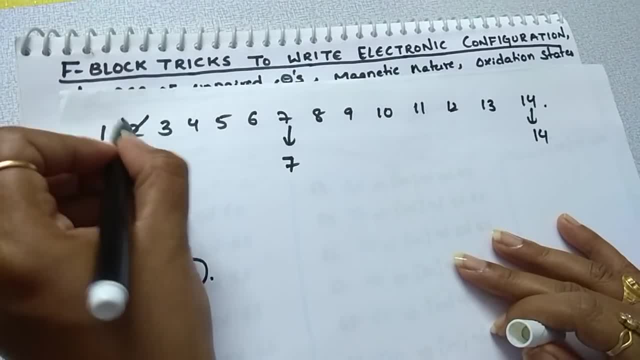 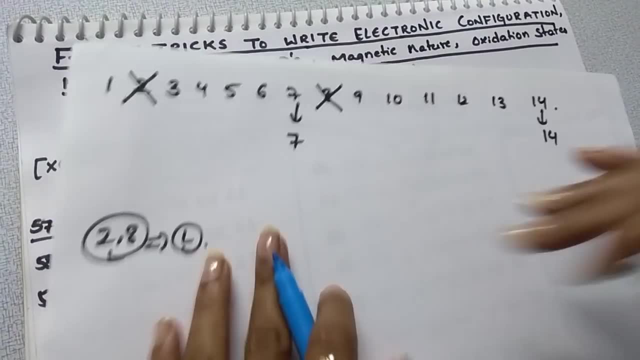 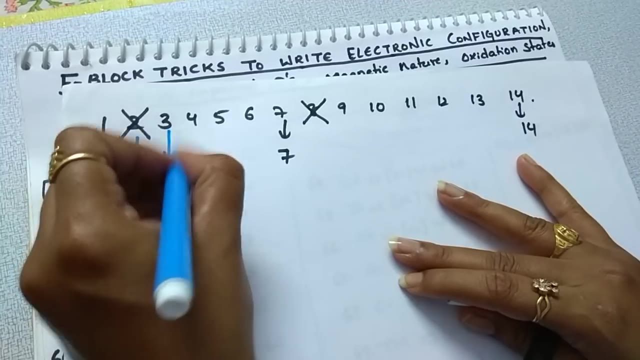 2 and 8 for lanthanates: Cross 2 and 8.. 1. Take as it is, Don't take 2. So take the next number 3.. Next number 4.. Next number 5.. Next number 6.. 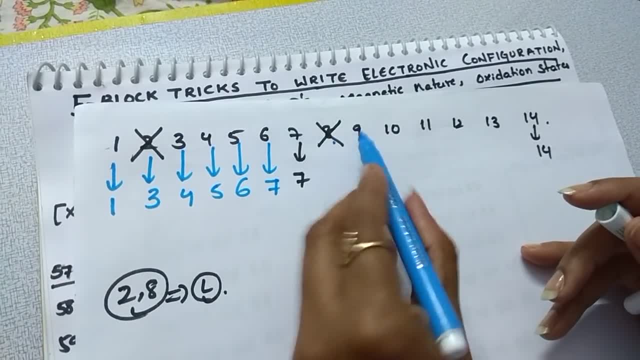 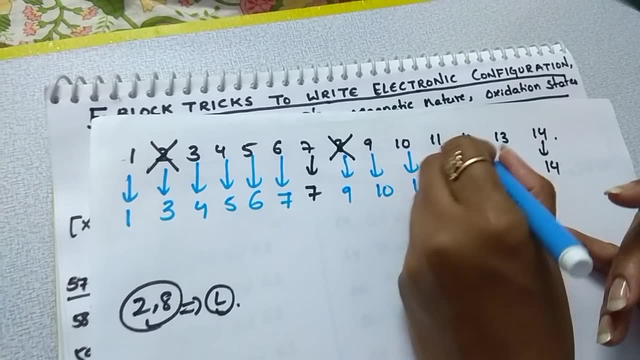 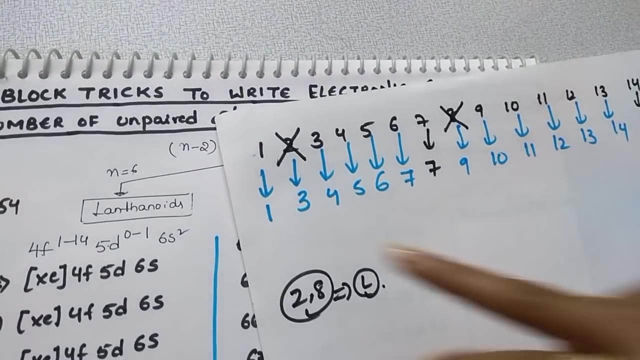 Next number is 7.. Don't take 8.. Next number: 9.. Next number: 10.. Next number: 11., 12., 13., 14. Right After writing this, just fill the electrons Cerium onwards. F block starts right. 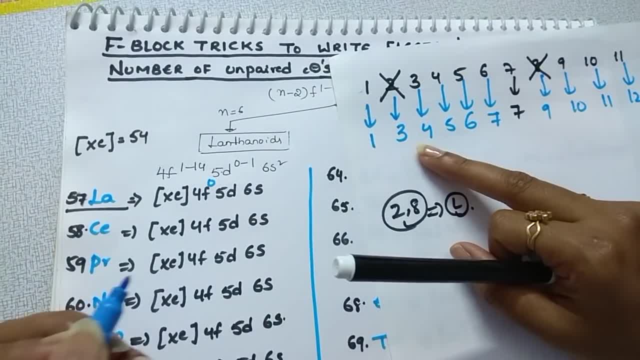 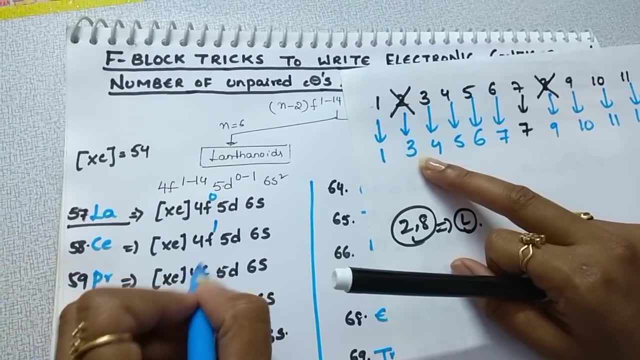 Lanthanum is not an F block element, It is a D. No electrons in F From cerium onwards. these are lanthanates F block elements. So fill 1., 3. Next, 4., 5.. 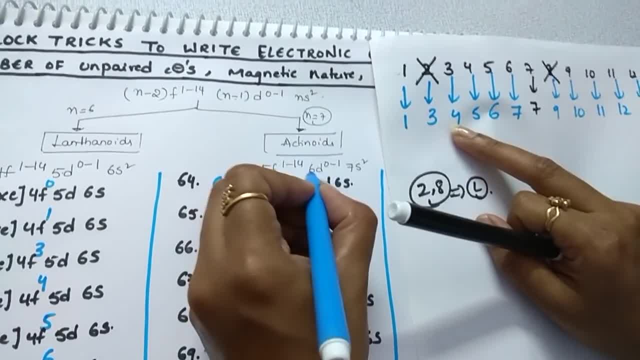 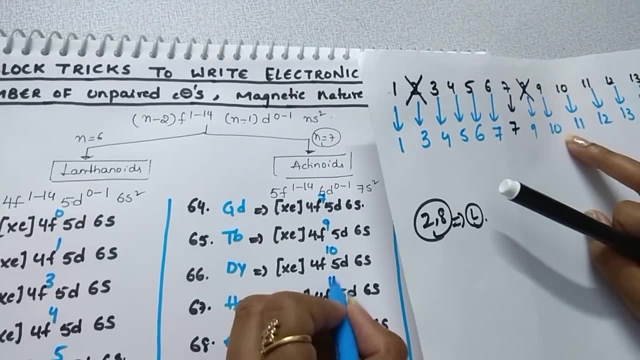 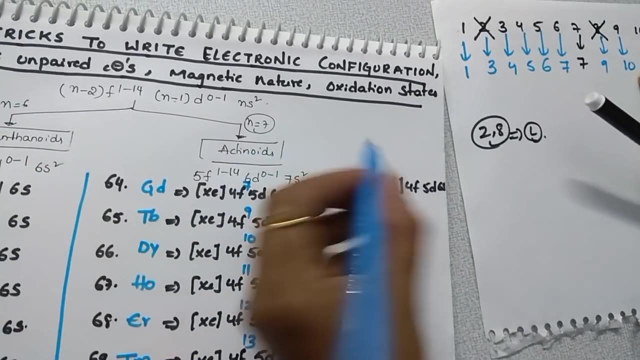 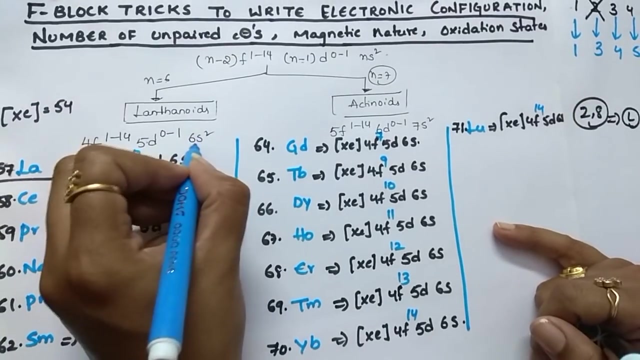 6., 7.. Fill 7.. Next, what is the number students? 9., 10., 11., 12., 13., 14., 14.. And after filling the F from these numbers, what you have to do is just see this. 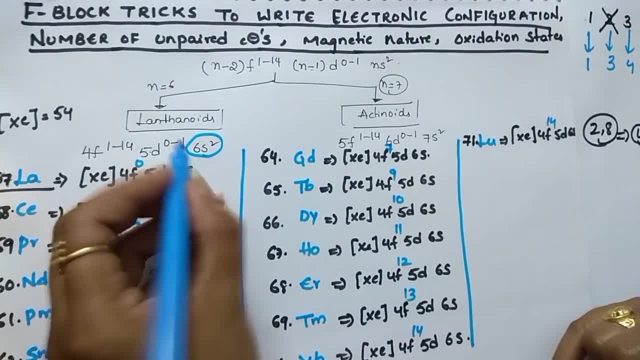 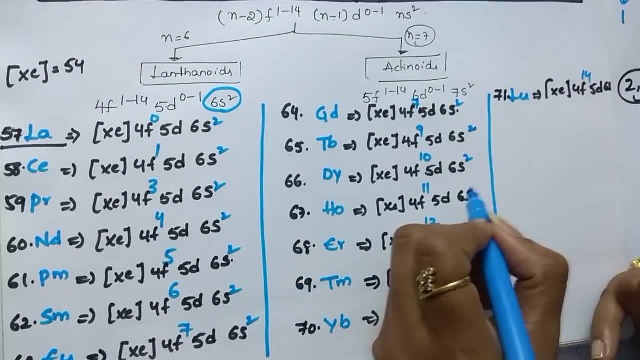 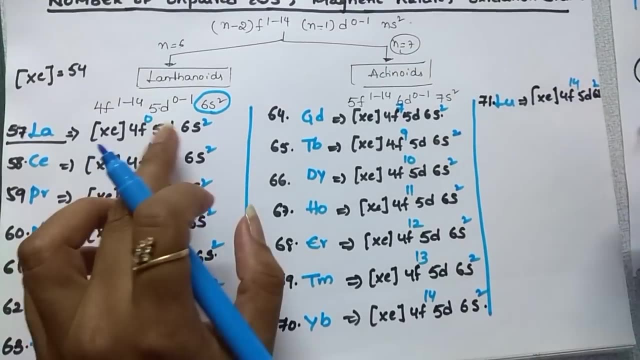 6 is 2.. S is completely filled. 2 electrons. No change in this. So fill this S orbital of all with 2 electrons. 2 electrons, Yes. After filling this S, what is left? D is left. 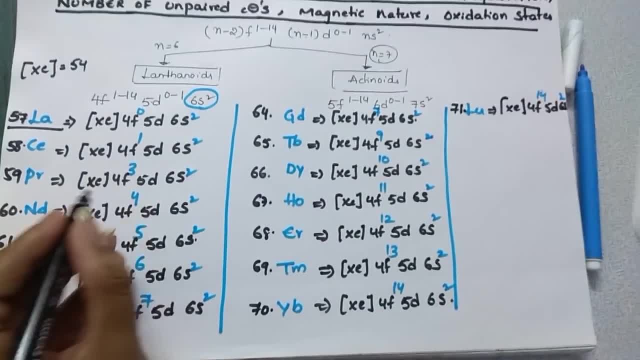 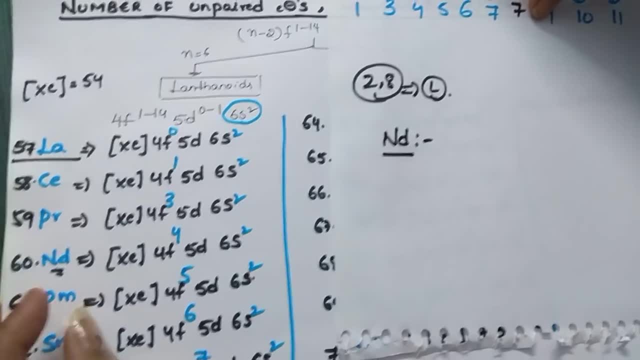 Listen carefully. What you have to do is suppose, take neodymium, You want to find the electronic, you want to write the electronic configuration of neodymium. What is the atomic number of neodymium? 60, right. 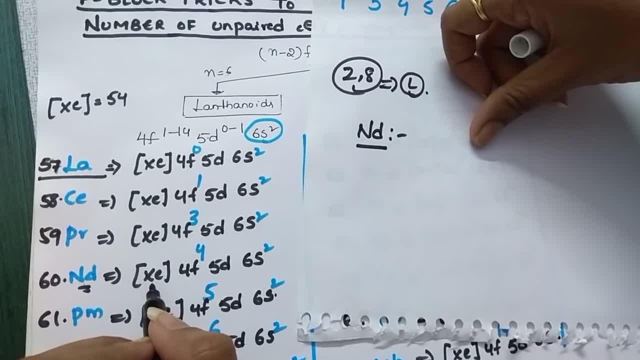 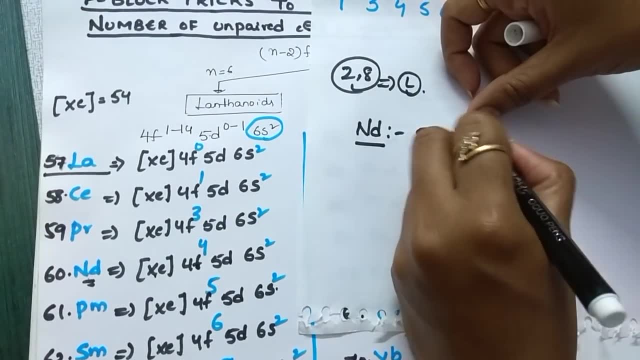 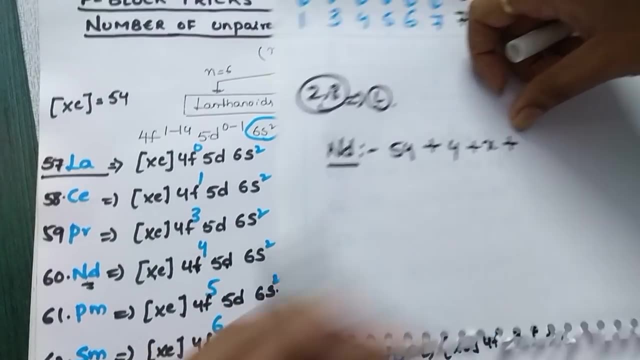 And how many electrons You filled already. xenon is 54 atomic number, So write that 54 plus F is having how many electrons? students, 4 electrons plus D. You don't know the number of electrons. Let us take it as X plus S is having how many electrons. 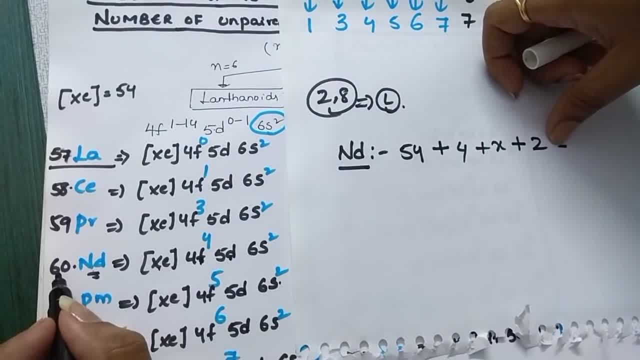 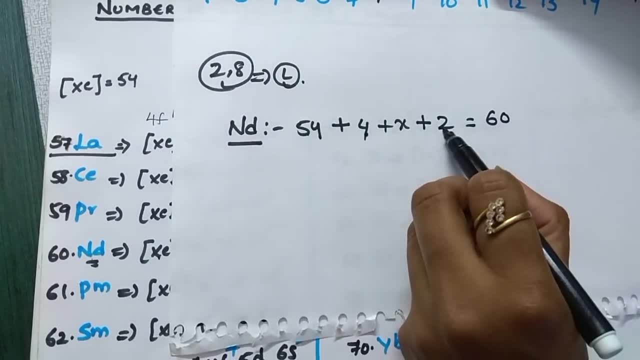 2. The total number of electrons should be equal to its atomic number, right, That is how much? 60.. 54 plus 4, 58.. 58 plus 2, 60. So X plus 60 is equal. 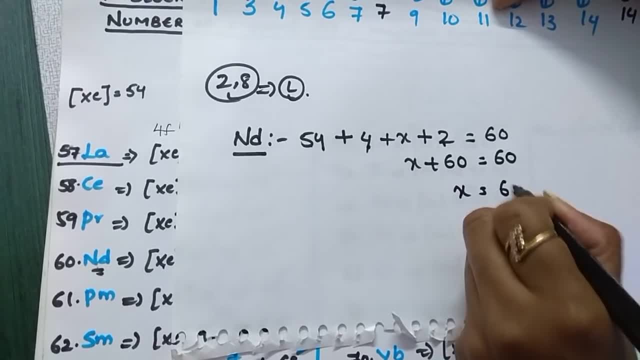 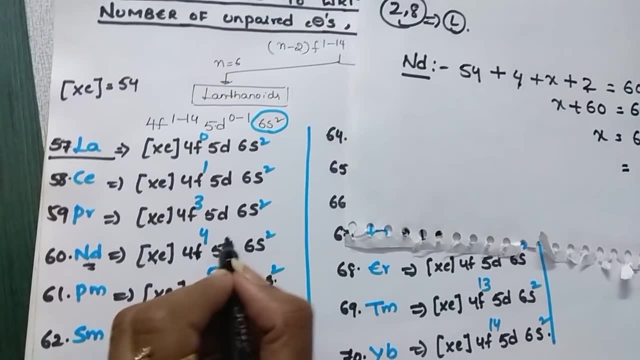 Then X is equal to, if it go this side, 60 minus 60, which is equal to 0.. Means the number of D electrons are 0.. Means there is no D electron. Fill that D 0. 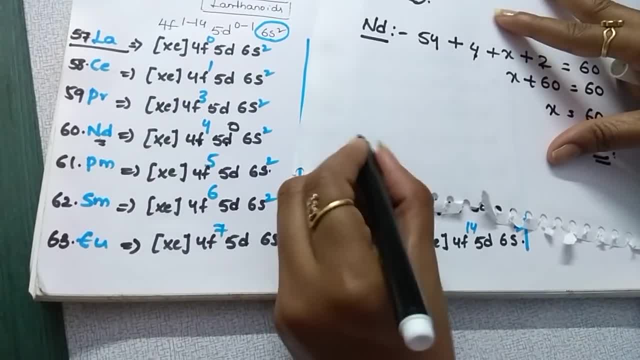 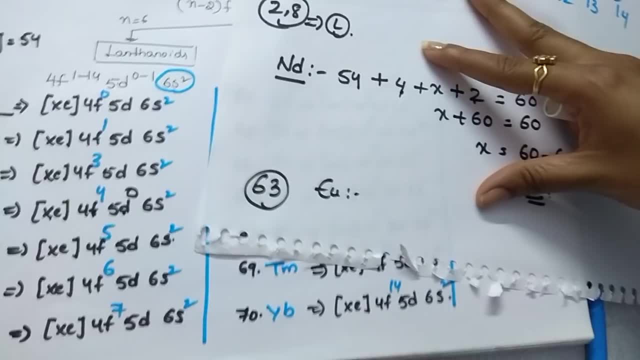 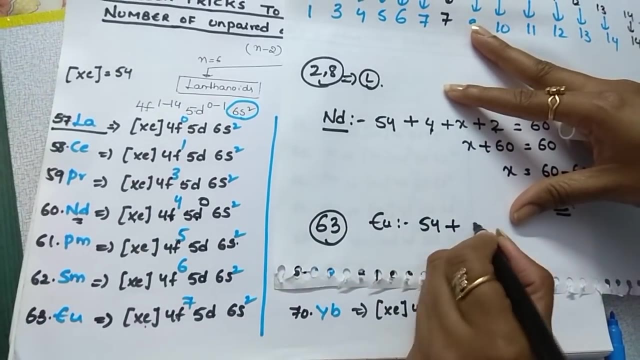 Take anything like europium. Europium atomic number is 63.. Correct, Europium. what you have to do, Xenon, you already Xenon, 54.. 54 plus 7 in F plus D, you have to find. 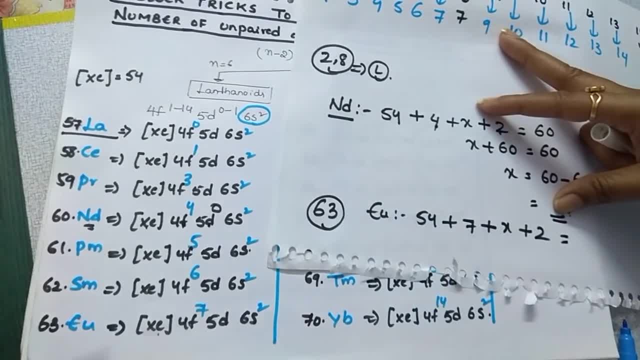 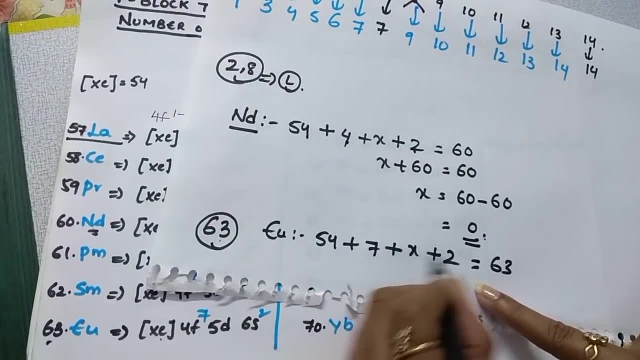 X, you don't know, S is 2.. Then the total should be equal to its atomic number, 63. Then 54 plus 7, 61.. 61 plus 2, 63. Means X is equal to 63 minus 63.. 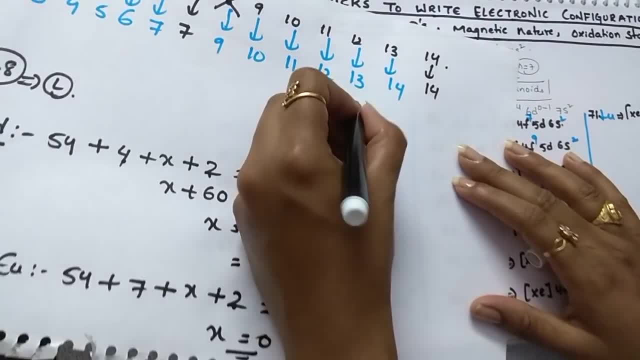 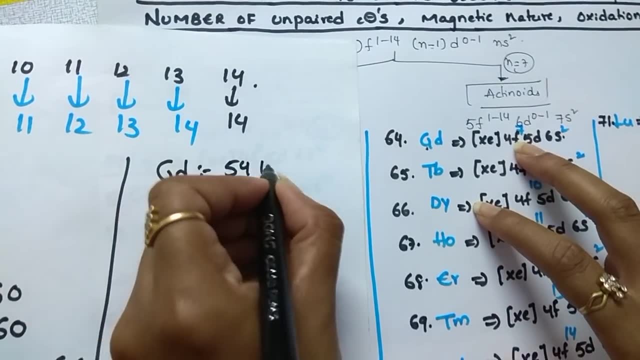 No electrons here. Let us see for gadolinium. you want to find Gadolinium? Xenon is 54. Plus already you filled 7 in F D. you don't know X Plus S is how many. 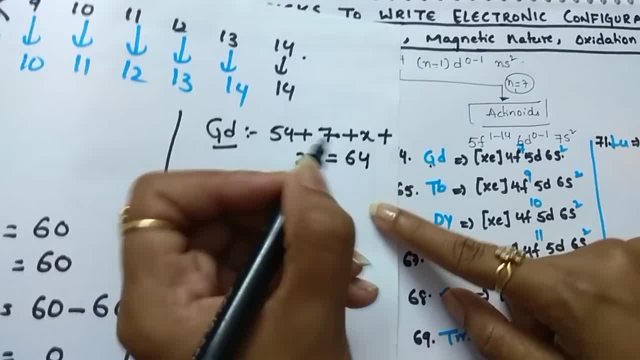 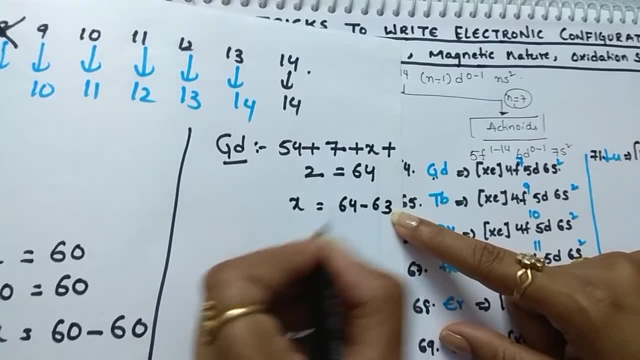 2. The sum is equal to its atomic number 64. Then X is equal to 54 plus 7,, 61 plus 2, 63.. 64 minus 63 is 1.. So the number of electrons in D is 1.. 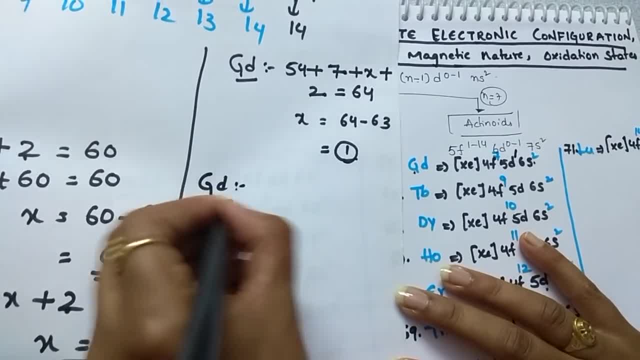 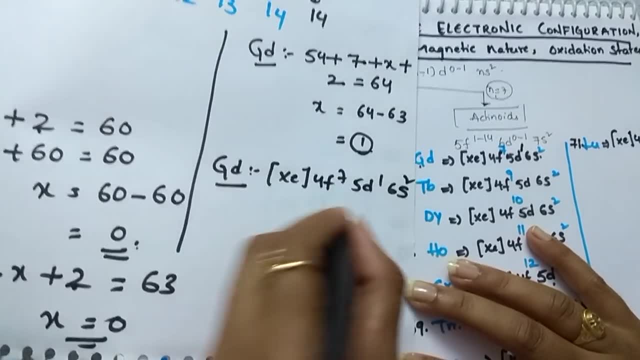 Now, what is the configuration of gadolinium? Xenon 4F7,, 5D1.. 5D1.. 6S2.. This is the electronic configuration of gadolinium. Just do it in this way. 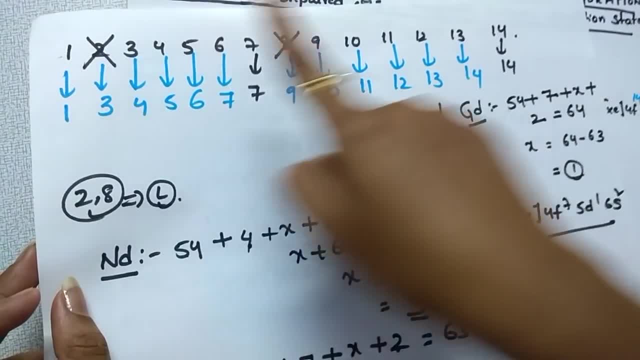 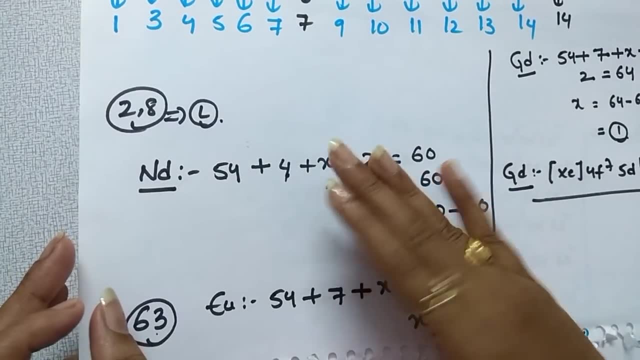 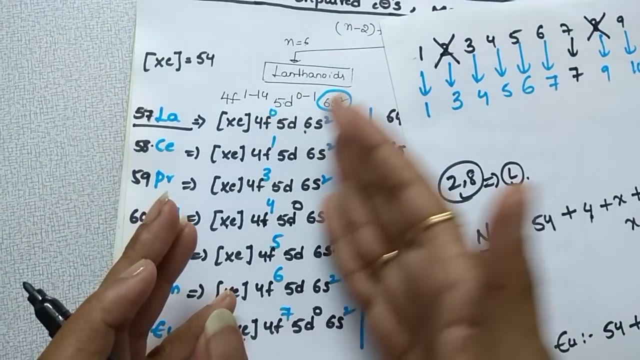 What you have to do? First strike off the numbers 2 and 8.. After that, take these numbers like this: Then fill these electrons in the F. After filling S also, you fill it. 2 to electrons, The total sum. add all the electrons and subtract this one from the atomic number. 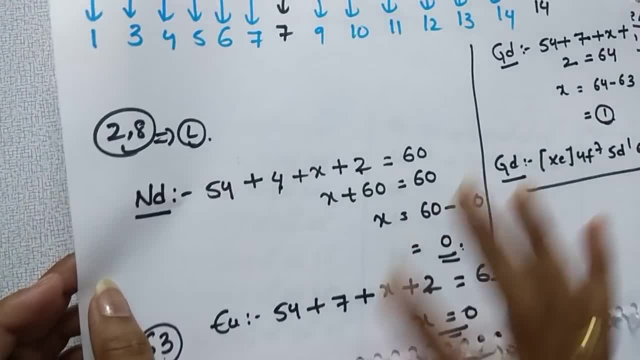 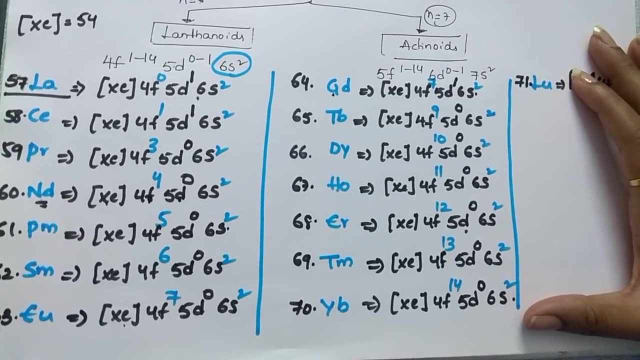 Then, whatever the number you get- That is the number of electrons in D After filling- you are going to get these electronic configurations And in my next video I am going to do about actinides. I am going to discuss about actinides. 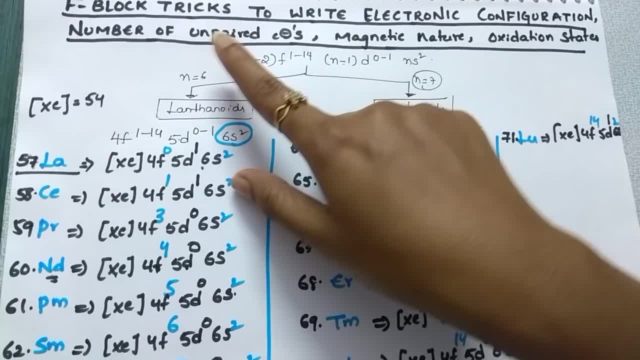 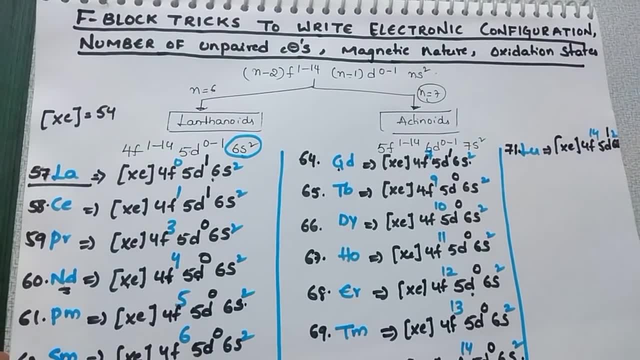 At the end of that session, I am going to discuss how to find the number of unpaid electrons based on that magnetic nature and oxidation states, which is more stable state and which one acts as an oxidizing and reducing agent. So don't miss that video. 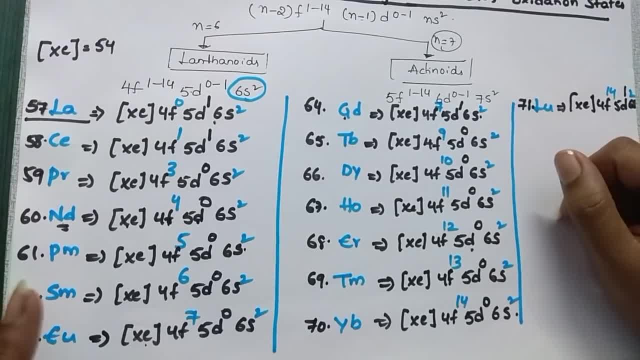 I hope you like this video. Please give thumbs up And thanks for watching. 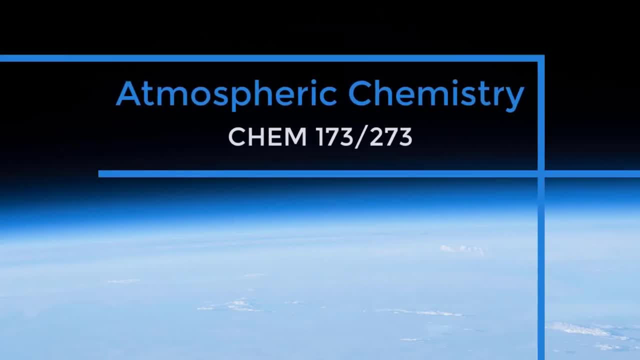 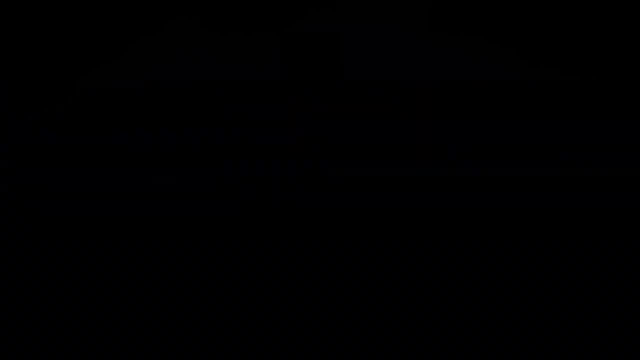 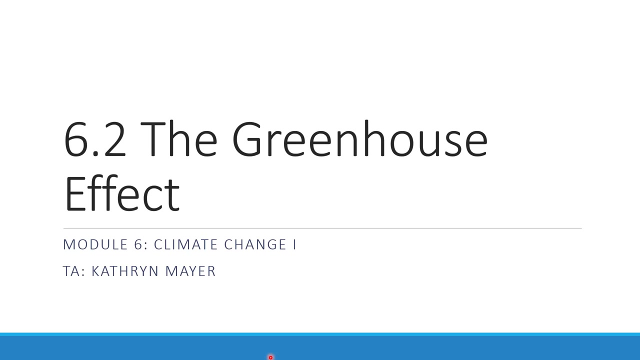 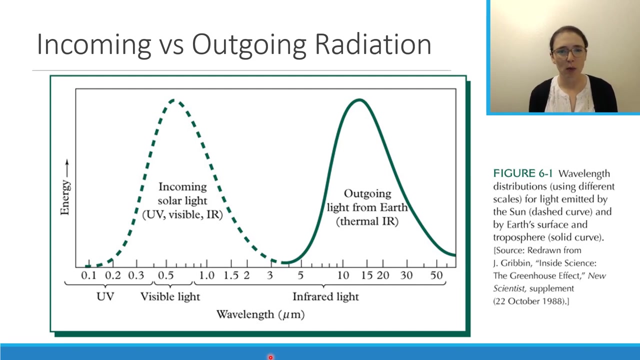 Hi everyone, welcome to lecture 6.2.. In this video I'm going to be talking about the greenhouse effect and the Earth's radiative budget, So let's review back to module 2, when we talked about radiation in the atmosphere. Remember that incoming solar light from the Sun is primarily